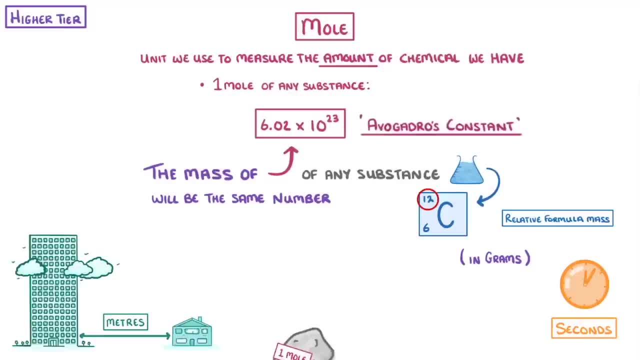 mass in grams. So our little pile of one mole of carbon would weigh exactly 12 grams, because carbon's relative atomic mass is 12.. Meanwhile, one mole of oxygen, which has the relative formula mass of 16 times 2,, so 32,. 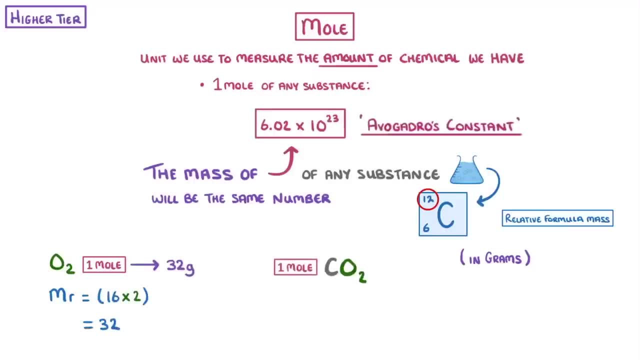 would weigh 32 grams. Or one mole of CO2, with a relative formula mass of 12 plus 16 plus 16, and so 44, would weigh 44 grams. But in all these cases there would be 6.02. 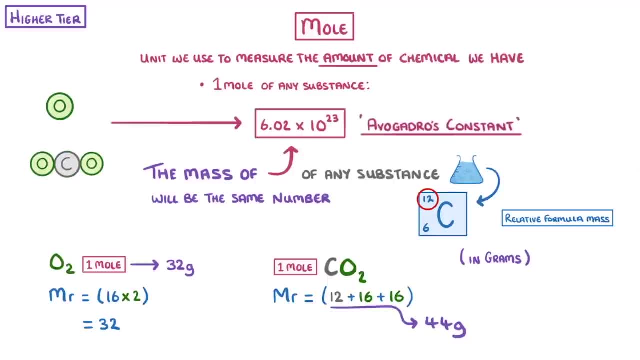 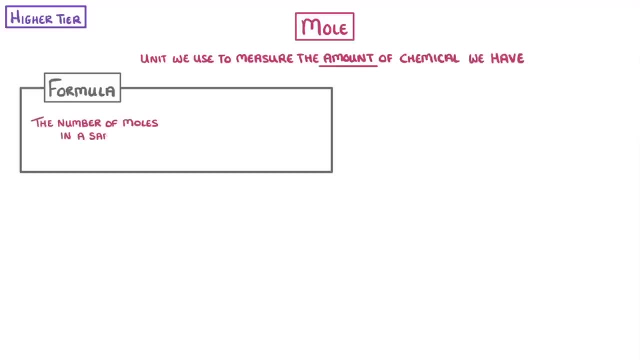 times 10 to the 23 atoms or molecules. Because of this rule, we can't measure the mass of any substance that contains 6.02 times 10.. We can create a formula which tells us that the number of moles in a sample is equal. 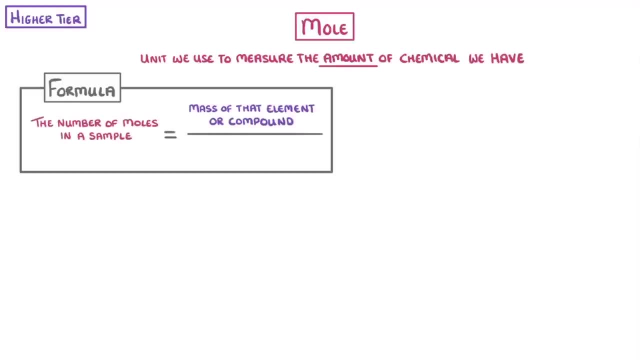 to the mass of that element or compound divided by its mR. So if we want to know how many moles there were in 42.5 grams of ammonia, we would do 42.5, which is the mass divided by 14, plus 3 times 1,, so 17,, which is the mR of ammonia, And this would give us 2.5. 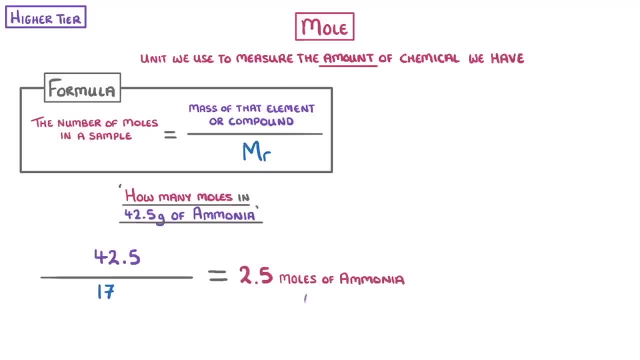 So we know that there are 2.5 moles of ammonia in the 42.5 grams. We can also rearrange the formula to find the mass. if we were given the number of moles, For example, what's the mass of 3 moles of carbon dioxide? Well, this time we'd multiply. 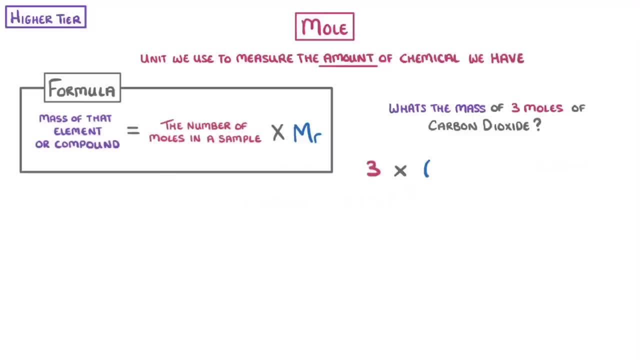 our 3 moles by the mR of CO2, which is 12 plus 2 times 16,, so 44,, which gives us 132 grams of CO2.. We can also work out the mass of a particular element within a larger compound. 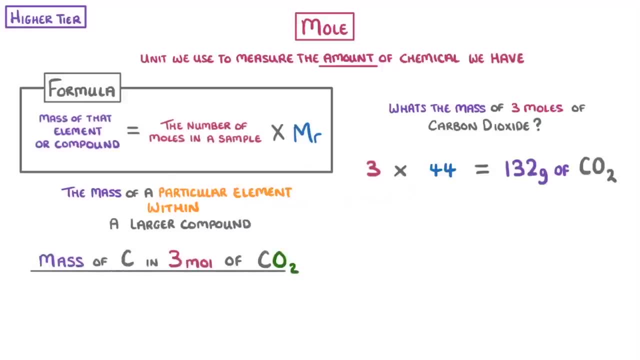 like the mass of carbon in 3 moles of carbon dioxide. For this, all we do is take the number of moles, which is 3, and multiply it by the mR of the carbon, which is 12.. So 3 times. 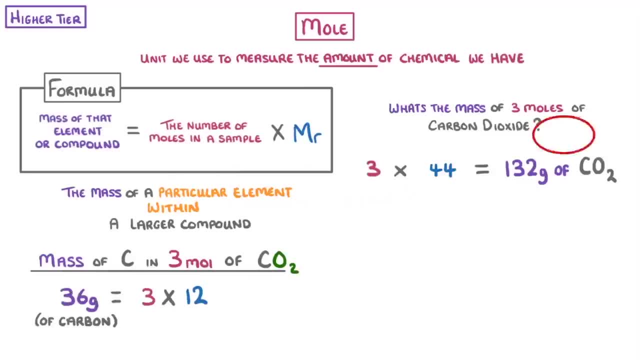 12, which gives us 36 grams of carbon in our 132 grams of carbon dioxide. If you wanted to go one step further, you could subtract that 36 grams from the original 132 grams to find that there must be 96 grams of oxygen, Because we can see that CO2 is.